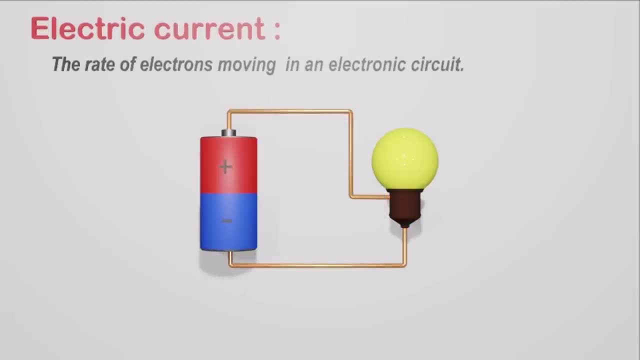 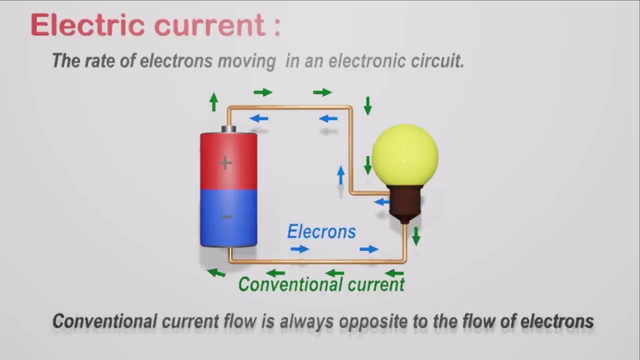 Even though the electrons flow from negative terminal to positive terminal. in most of the textbooks, conventional current assumes that current flows out of the positive terminal through the circuit and into the negative terminal of the source. This was the convention chosen during the discovery of electricity. It was not quite accurate. 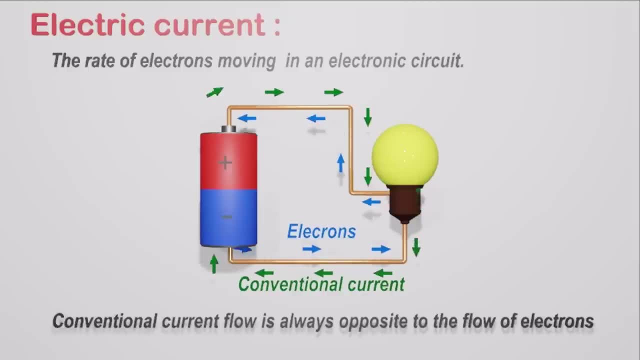 We have unfortunately stuck with this convention to this day, and so current flow from positive to negative is called conventional current flow and is used when drawing circuits. In fact, it makes no difference which way current is flowing, as long as it is used consistently. 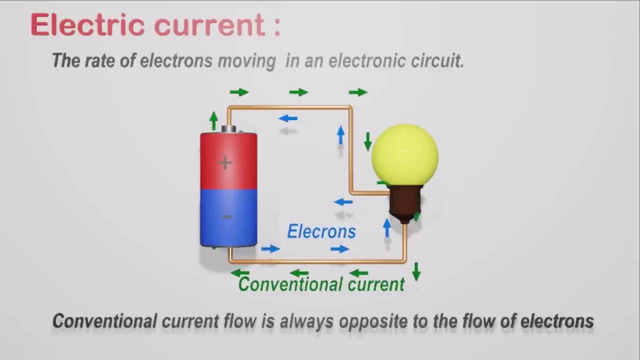 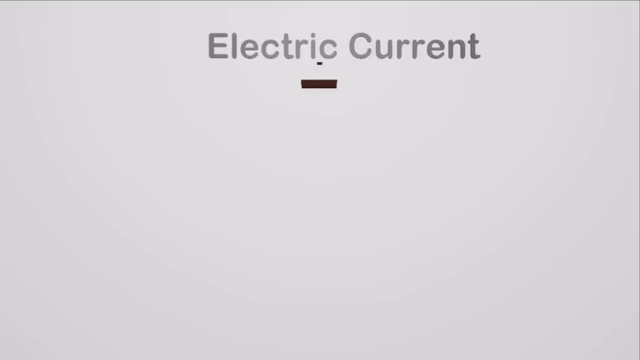 The direction of current flow does not affect what the current does. Throughout this video, we use the term current for the conventional current. There are two forms of electric current: Alternating current- AC- and direct current- DC. One is not better than the other, as both are necessary. 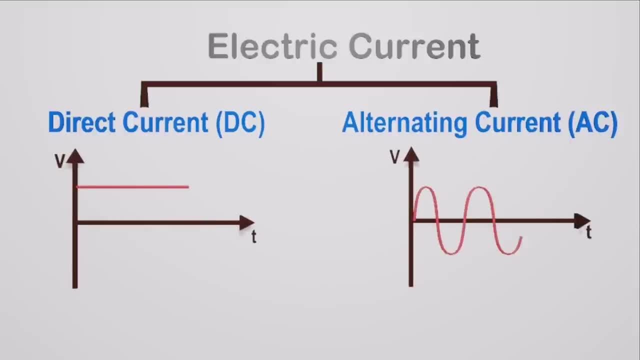 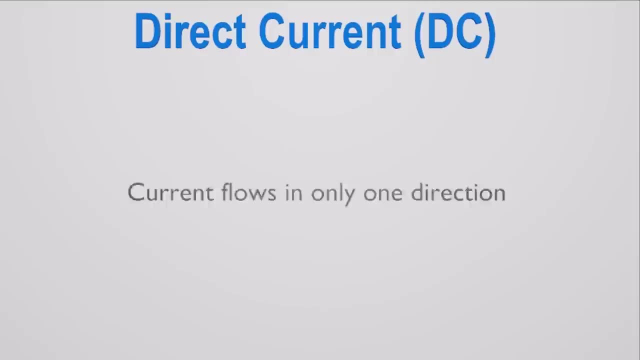 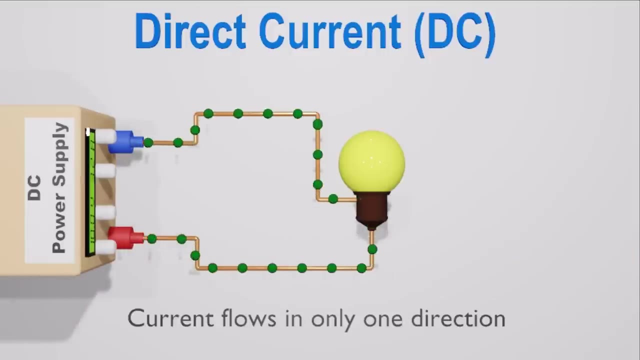 Here we will explain each of them and how to convert direct current into alternating current. Lets start with direct current. DC is a linear type of electrical current. Direct current always only flows in one direction: From positive pole to negative pole. Keep in mind that the electrons flow opposite to that. 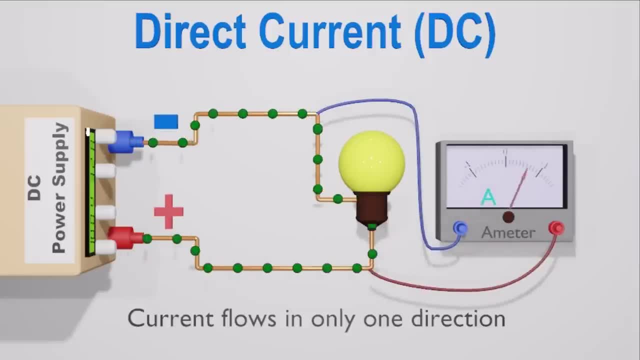 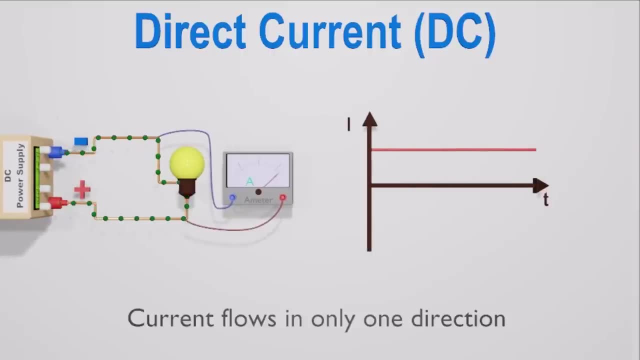 For DC, the positive and negative poles always remain the same. We can draw a graph for the magnitude of direct current with the time like this: since the current is then does not flow in the opposite direction, the graph only has a positive side. dc powers appliances. 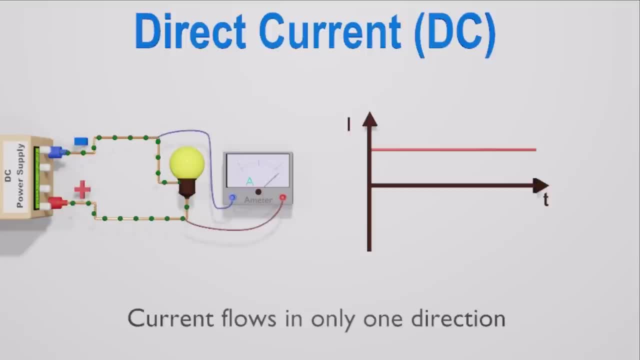 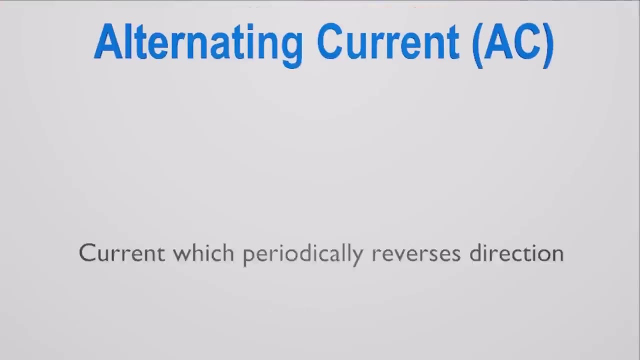 with delicate electronic circuits that require a simple and steady current flowing in one direction. nowadays, this type of current powers cell phones, computers and most other electronics and the current obtained from batteries, solar cells, etc. how does ac work? alternating current? ac is an electric current which periodically reverses direction and changes its magnitude. 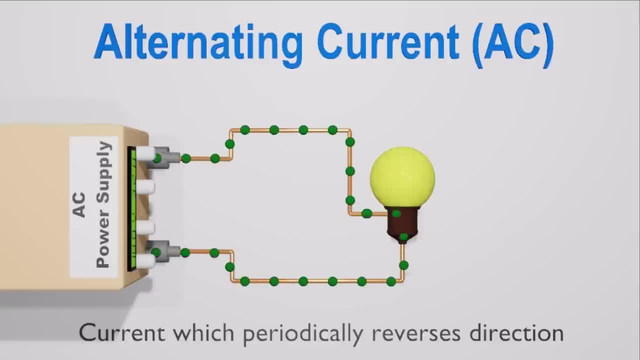 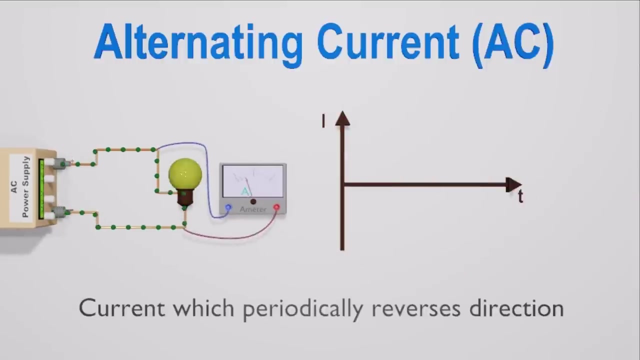 continuously. with time, ac constantly changes its flow between positive and negative terminals. this means that electrons also change their flow following the negative to positive end as the polarity changes. we can draw a graph for the magnitude and direction of alternative current with the time like this, since the current changes its direction. 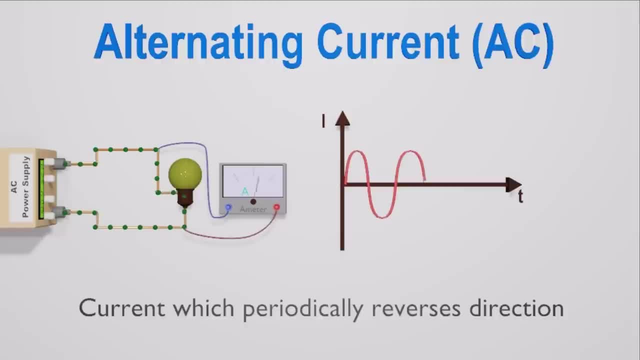 periodically. the graph has both positive and negative cycles. the speed at which ac changes polarity and completes several cycles in one second is called frequency, and it is measured in hertz. the most common ac waveform that is used in electrical and electronic engineering is the sinusoidal waveform. however, an alternating ac waveform may not always take the shape of a smooth. 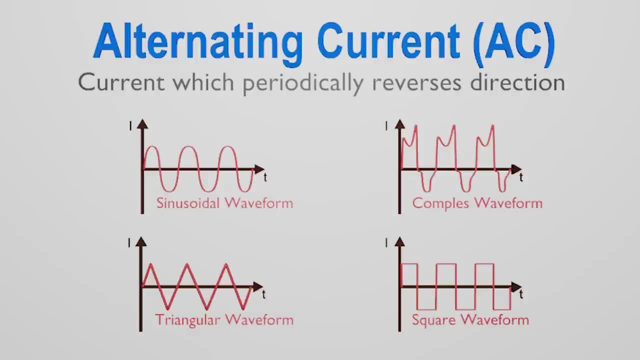 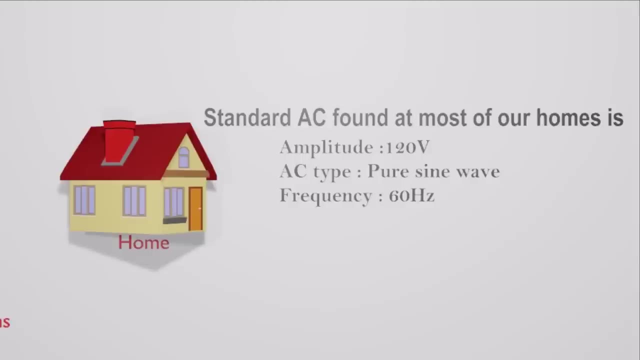 shape based around the trigonometric sine or cosine function. ac waveforms can also take the shape of either square waves, triangular waves or any other complex shape. standard ac found at most of our homes as a 120 volts amplitude pure sine wave with a 60 hertz frequency. however many 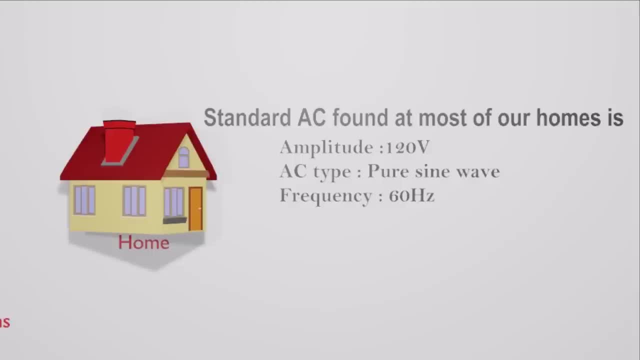 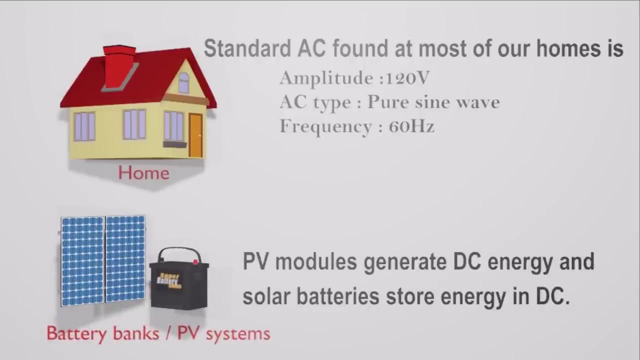 appliances and electronics use direct current, dc, which provides consistent power to the device. we explain how to convert ac into dc in our previous videos. on the other hand, most renewable power generation systems, such as solar pv systems and wind generators, involve dc, so it is important to convert this generated dc into ac for. 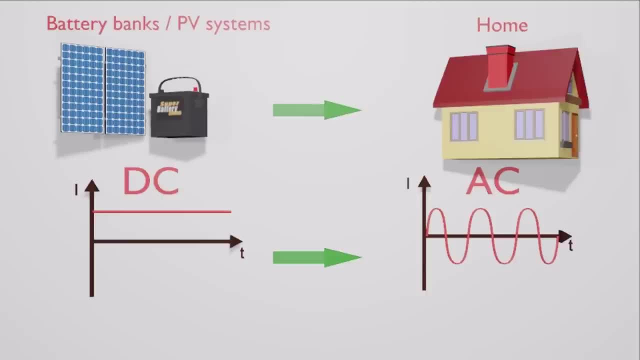 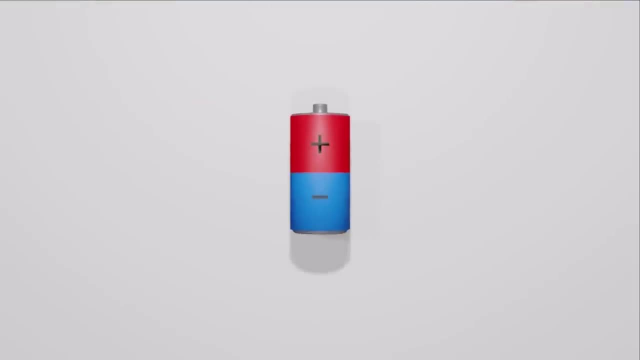 distribution purposes. in today's video we are going to talk about how to convert dc to ac or inverting the dc. just imagine you have a dc battery that can supply direct current and someone taps you on the shoulder and asks you to produce a c instead. how would you do it if? 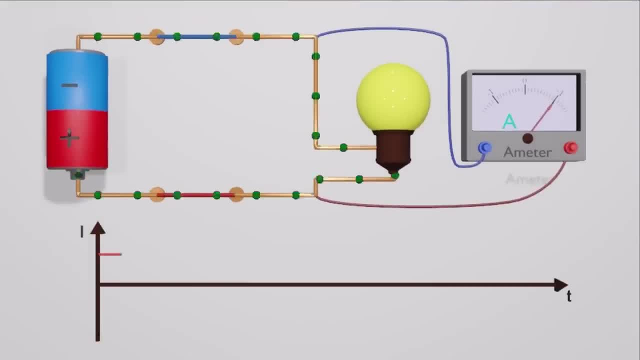 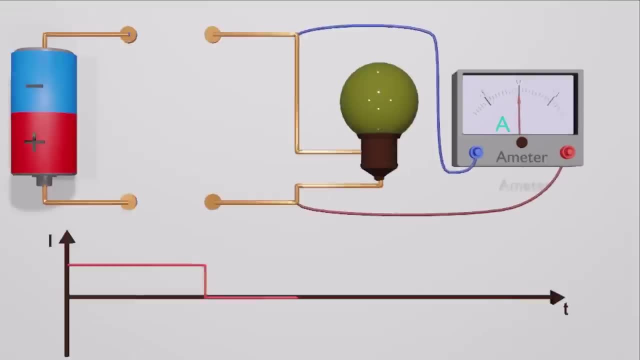 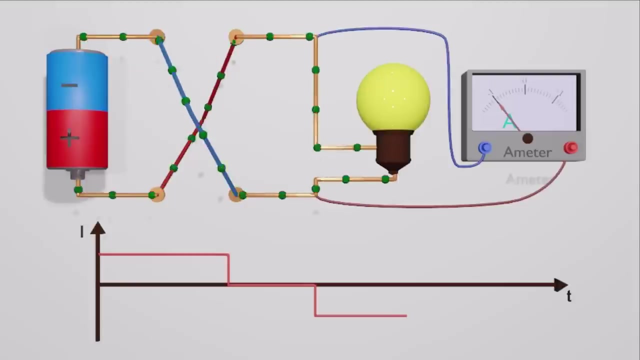 all the current you produce flows out in one direction. what about disconnecting the wires? the current becomes zero. then let's flip it back. now we have current that flows in the opposite direction. likewise, we can change the wires back and forth, so the current direction keeps reversing. 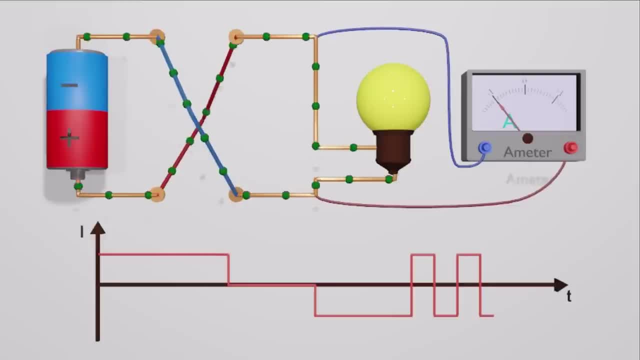 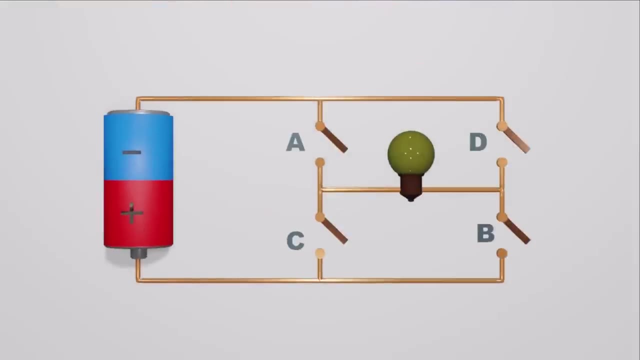 what you end up with is very abrupt changes of current, all in one direction, all in the other direction and back again. look at the graph of the current. you'll get a square wave, although electricity varying in that fashion. technically it's an alternating current. instead of swapping the wires, we can do this by using four switches. 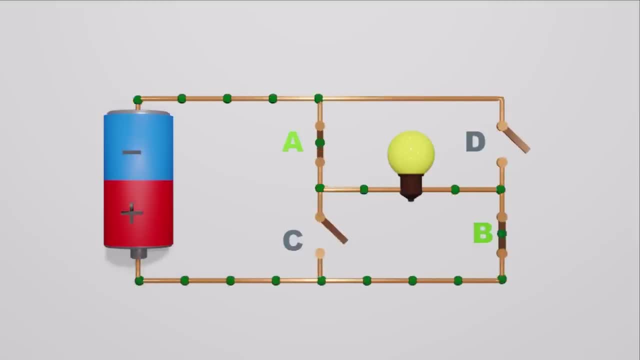 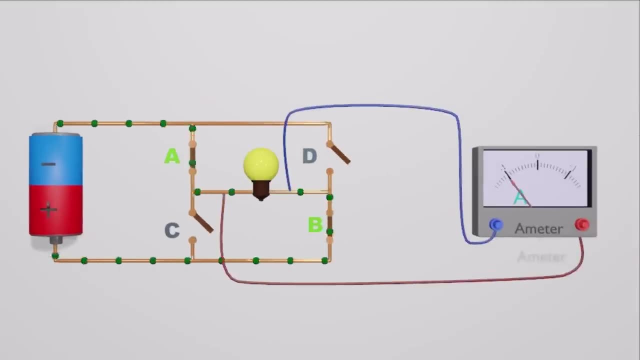 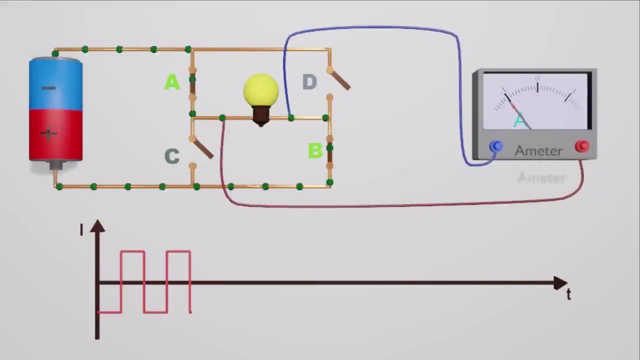 switching your current in given manner on and off very rapidly would give pulses of direct current. we called this as h bridge arrangement, which would do at least half the job. to make proper ac, you'd need a switching h bridge arrangement that allowed you to reverse the current completely and do it about 50 to 60 times every second. 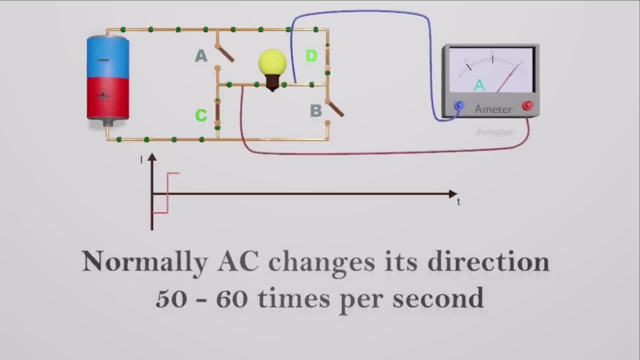 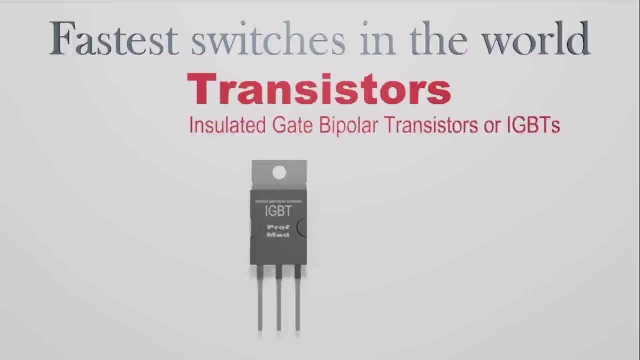 visualize yourself swapping your switches back and forth over 3000 times a minute. that's some neat finger work you'd need. that is why we use the fastest switches in the world- transistors. we can use transistors more specifically: insulated gate bipolar transistors or igbts. 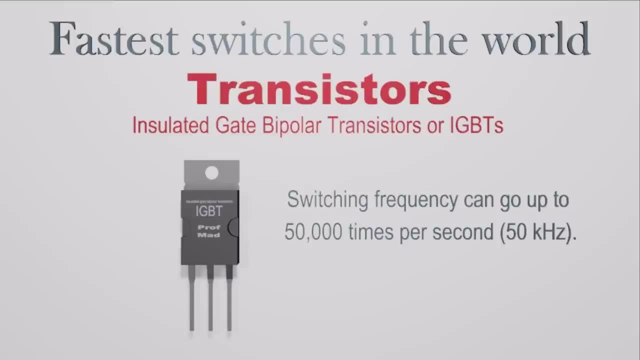 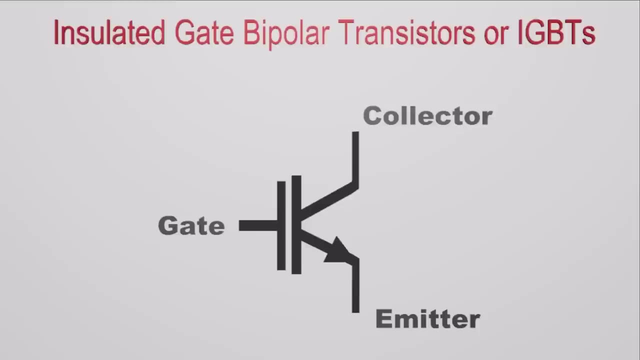 most common igbt switching frequency ranges from 20 to 50 kilohertz. an igbt is a three terminal power semiconductor device primarily used as an electronic switch. igbt can be switched on and off by activating and deactivating the gate. if we make the gate more positive by applying 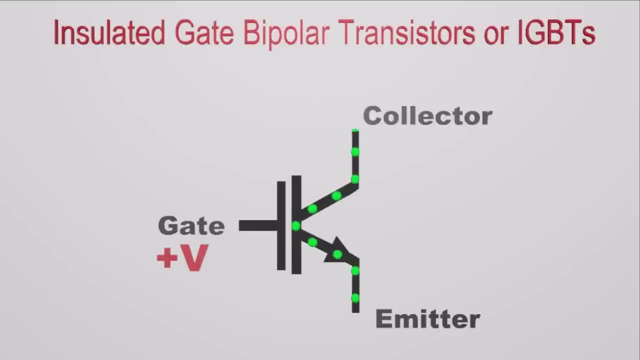 an chip to the gate, the partido current can flow from the collector to emitter. so the igbt in its almost zero on state. if we make the gate negative or zero, the current can flow from the collector to emitter. the current flow stops and IGBT will remain in off state. 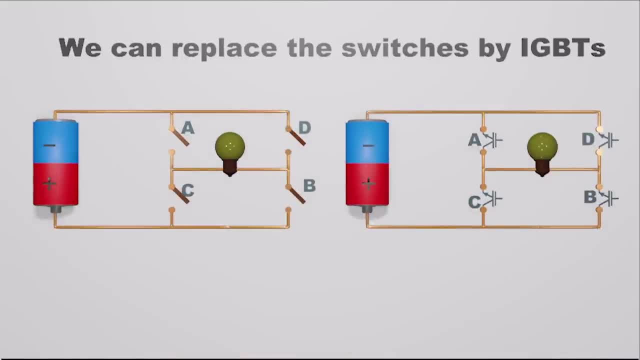 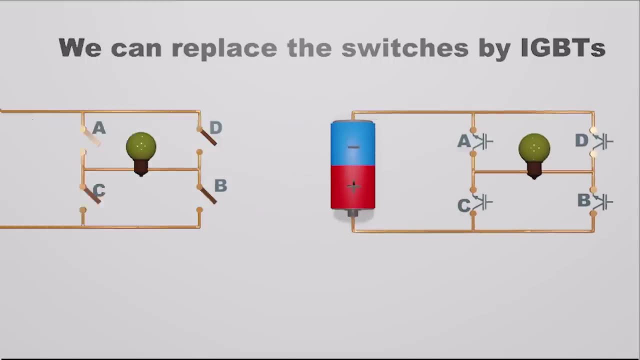 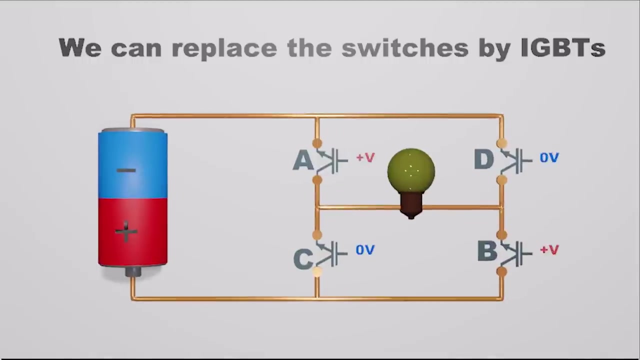 We can use IGBTs as switches. At its simplest, an inverter consists of what is known as a H-bridge arrangement. This circuit illustrates the implementation of a single-phase H-bridge circuit using four IGBTs. The operation of the H-bridge is straightforward: By closing A and B. 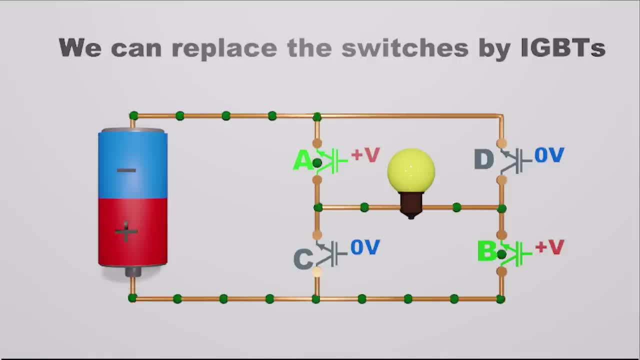 and opening C and D at the same time, current starts to flow through the bulb from left to right. By opening A and B and closing C and D at the same time, current starts to flow through the bulb from right to left. Likewise, by turning on and off the IGBT switch pairs, reverses the 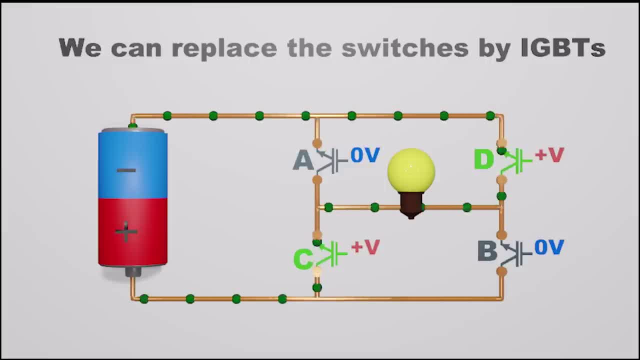 current direction- That means alternating current- is generated. To work these IGBTs correctly, we can use a switch to turn on and off the IGBT switch pairs. To work these IGBTs correctly, accurate control signals must be provided to A, B, C and D. 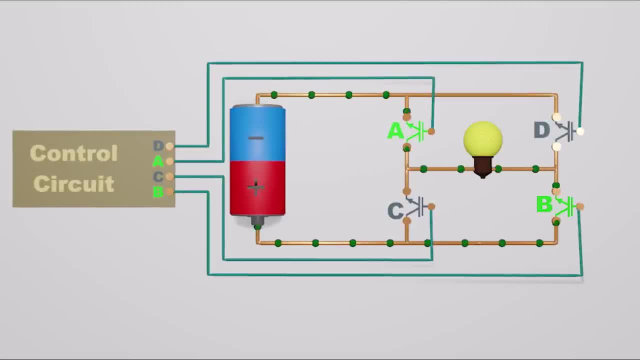 These control signals are generated by a separate circuit which can control the frequency of the output AC signal. As an example, we can use a cheap Arduino board to supply these controlling signals. Even though we converted the DC to AC square wave, it's not at all like the AC. 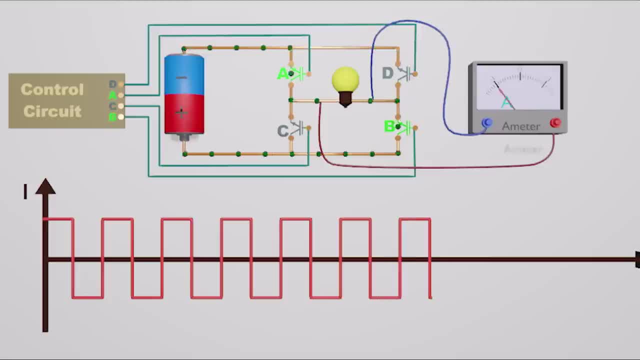 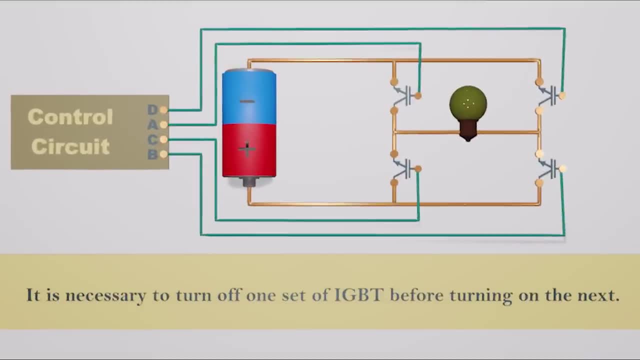 sine wave supplied to our homes, which varies much more smoothly. To avoid damaging the IGBTs at short notice, we can use a switch to turn on and off the IGBT switch pairs. This way we can use a switch to turn on and off the IGBT switch pairs. When changing polarity it is necessary.